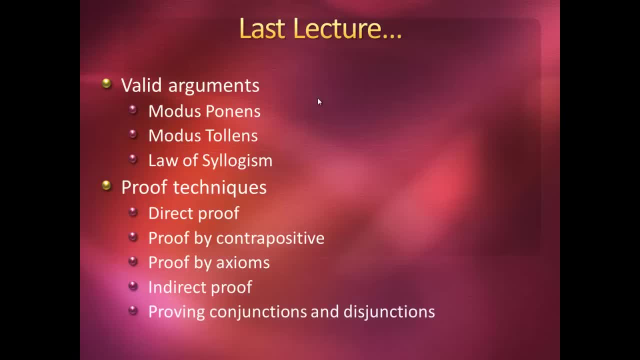 each one separately, and disjunctions split up the problem into cases or assume one thing is false and prove the other is true. Finally, we looked at biconditionals and saw that they can be split into two conditionals that can each be tackled separately. 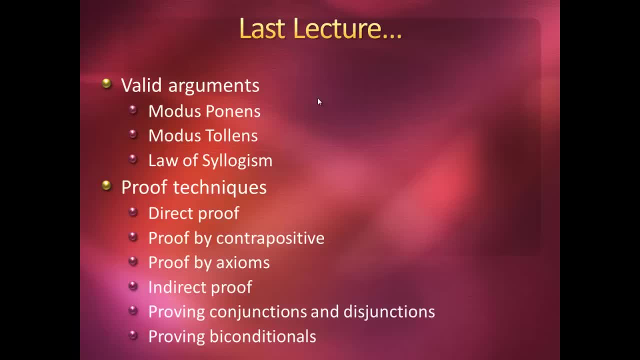 So we talked about logic, how we think, and proofs- how we can use that logic. If mathematics were a game, then so far we've learned the rules and learned some strategy. Now it's time to look at the playing pieces and get into one of my favorite topics. 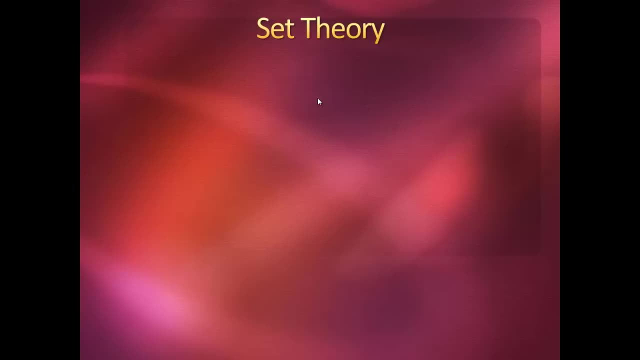 Set theory. Set theory was developed by German mathematician Georg Cantor. Technically, he wasn't the first to consider sets, as mathematicians dating back as far as Aristotle in ancient Greece had already been toying with the ideas we'll be seeing here. But it was Cantor who really gave it a firm footing. In particular, 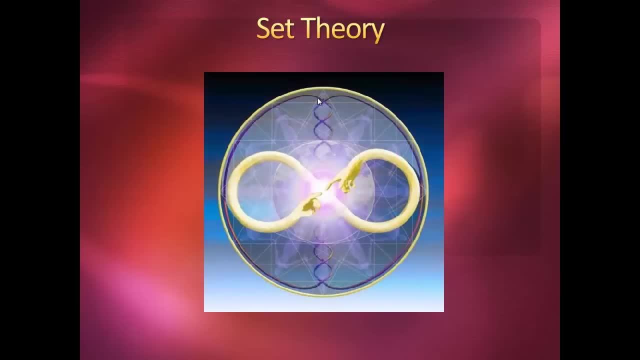 Cantor developed set theory to answer questions about different kinds of infinity, something that had been bugging mathematicians for a long time. We'll be dealing with the different kinds of infinity much later in the course. For now, we'll just be focusing on the beginnings of set theory. 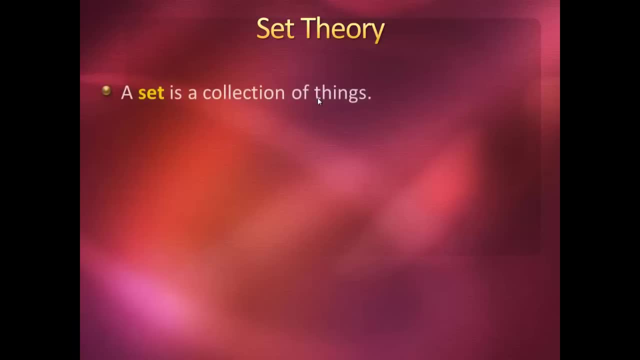 So what is a set? in its most basic sense, A set is a collection of things. What sorts of things? Well, just about anything. Of course, in math, you first would think of putting numbers in your sets, And of course that's what we often do, But by no means are you. 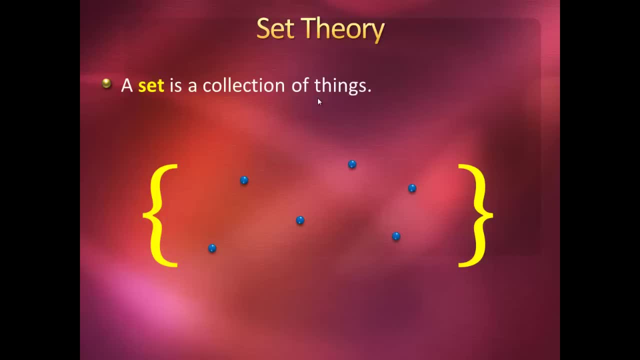 limited to this. You can have a set of points. By this definition, a line would be a set. You can have a set of people. You can have a set of colors. You can have a set of rules. Basically, think of a set as a box that you can fill with just about anything you desire. 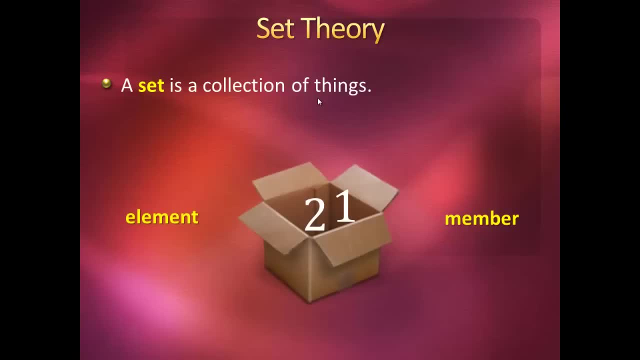 Each thing in the set is called an element or member of the set. Rather than drawing a bunch of boxes, though, we have a simple and compact way to represent a set. We use these little curly braces. So a set containing the numbers 1,, 2,, 3,, 4, and. 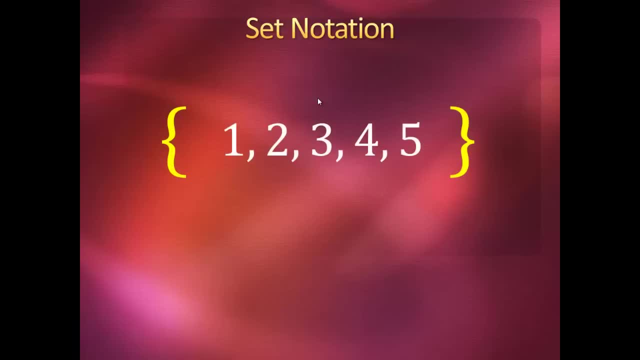 5 would be written like this. This way of writing a set is called roster notation. It explicitly lists out every element in the set. By the way, we usually represent sets with capital letters, So we might call this set A. Now I might give you a number, say 3, and ask you: is 3 in set A? Well, absolutely. 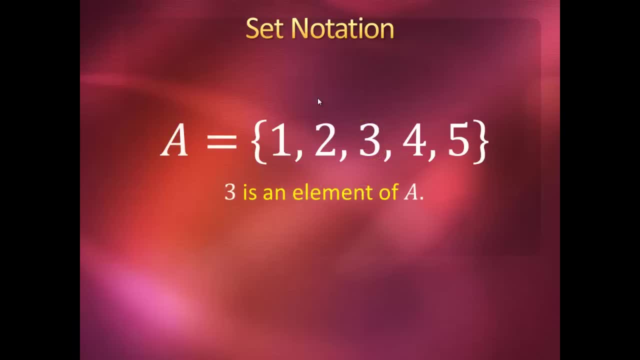 It's right there in plain sight. So we say 3 is an element of A. We have a special symbol we can use to say this: It's a little e, or actually the Greek letter epsilon. So when you see this, you say 3 is an element of A. 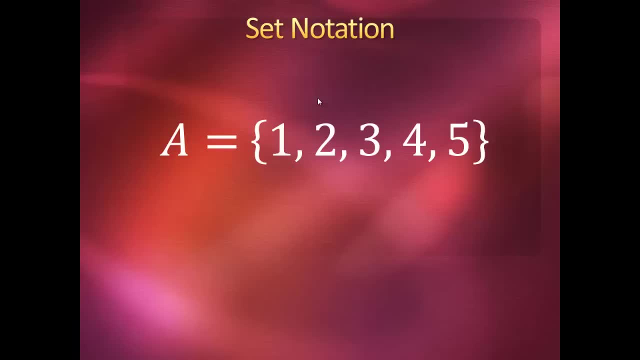 Now what about 6?? Is 6 an element of A? No, it's not, because A only contains 1 through 5.. So, as we would say and write: 6 is not an element of A. You just write the epsilon. 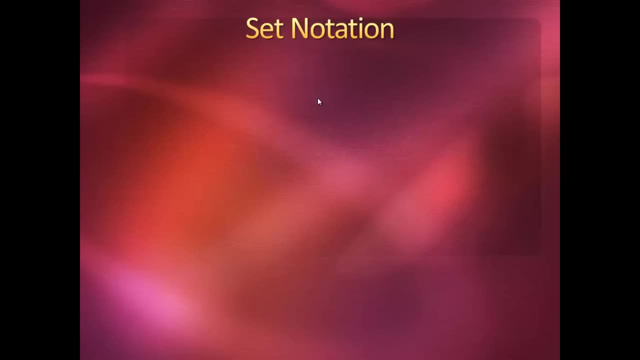 with a slash through it. If we want to refer to an arbitrary member of a set, we usually use a lowercase letter to match our uppercase letter. So we would say that little a is an element of big A. Two things to keep in mind about sets, by the way. First of all, in a regular set, an 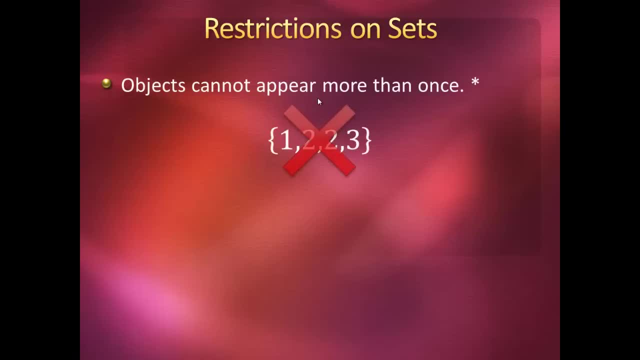 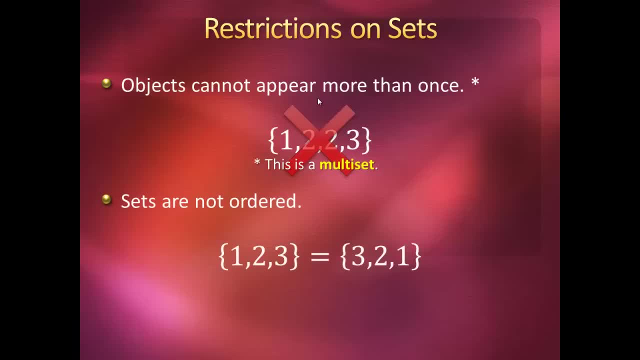 It's a set. It's a set. It's a set. The set 1, 2, 3 is the same as the set 3, 2, 1.. The only thing that defines a set is what's in it, not where each thing is. Like I said earlier, 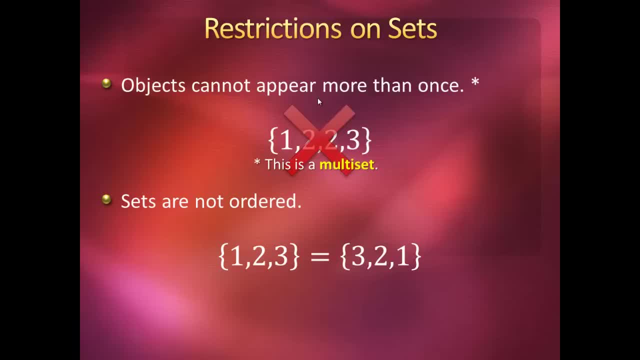 just think of it as a box, not necessarily a list. Now for smaller sets. roster notation is an easy means of representation. If you have larger sets, though, it becomes tedious, and if you have infinitely large sets it becomes impossible. For instance, what if I wanted to write the set of all, even integers? 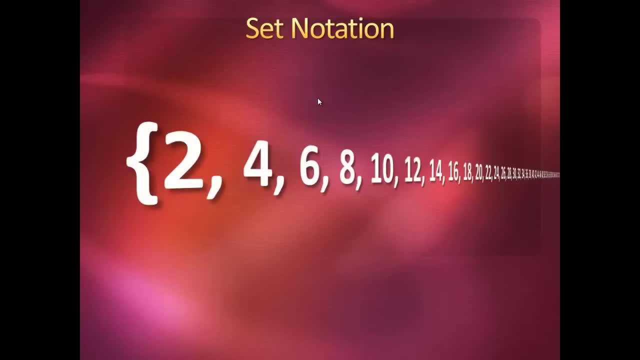 I don't want to write all of them down, that would take me forever. and then some. Luckily for us, there's another notation we can use for sets, called set builder notation. In set builder notation, rather than simply listing each element, we look at what sorts 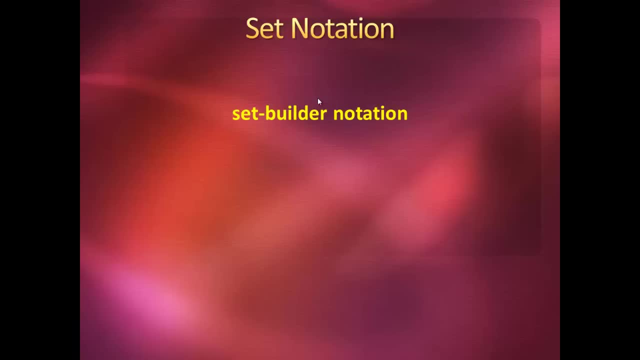 of things we want in the set, that is, what properties each element should have. So my set A from earlier could be written like this: We'd read this as the set of all x, such that x is an integer between 1 and 5, inclusive. 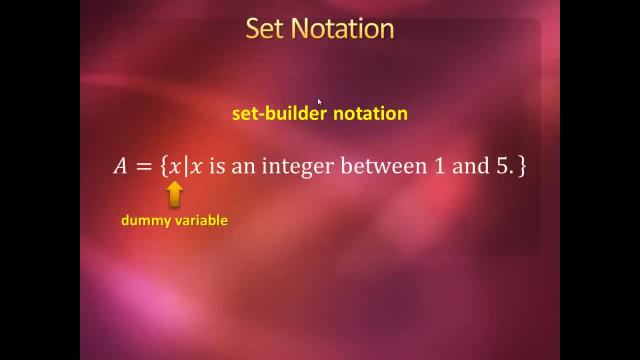 By the way, the x on the left is what we call a dummy variable. We don't have a particular reason for calling it x. We could have said the set of all y, such that y is an integer between 1 and 5.. 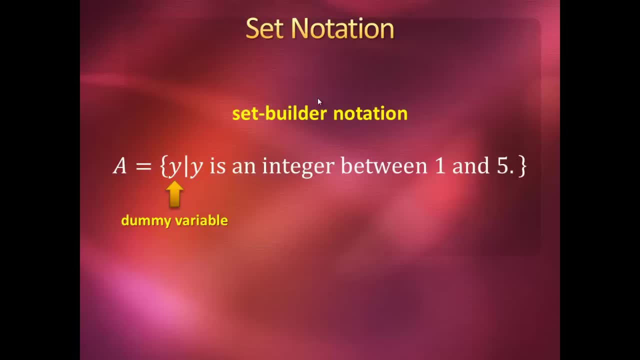 The x or y is only there, so we can use it to search for the numbers with the properties we want. We might more accurately say the set of all numbers that are integers between 1 and 5. So that's most of what we can do with only one set. 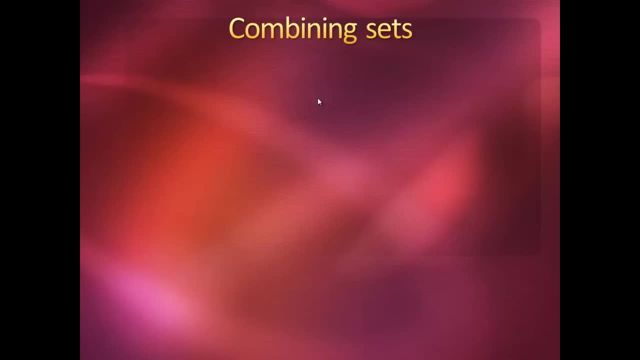 But, like in logic, things start to get interesting when we combine two or more sets in some meaningful way. So we've got some new symbols we'll use. Remember in logic we called these connectives, but in general when we have symbols that, 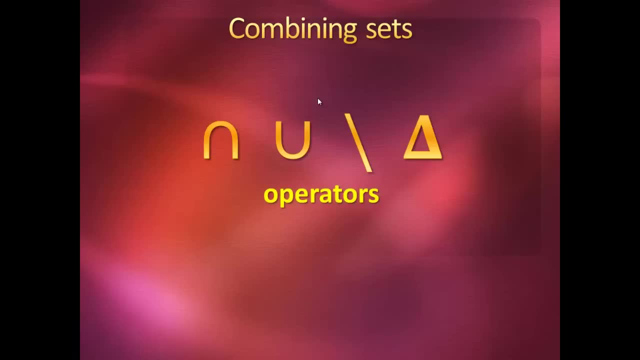 act on numbers or variables. we call them operators. So set theory has its own operators that we'll use. The first operator is called the operator. It's called the intersection. It's written like an upside down u, So we'd call this the intersection of a and b. or we might say out loud: a intersect b. 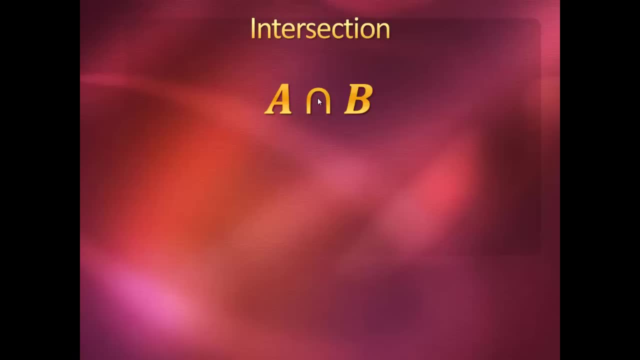 for short, To find the intersection of two sets. we look for what elements the sets have in common and put all those elements in another set. So let's use the set a equals 1,, 2,, 3,, 4, 5 from before and we'll make a new set b. 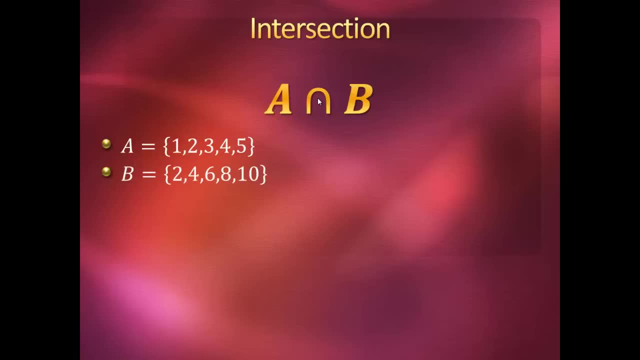 which will be 2,, 4, 6,, 8, 10.. So what numbers do a and b have in common? We've got 2 and 4.. So the intersection of a and b is the set 2, 4.. 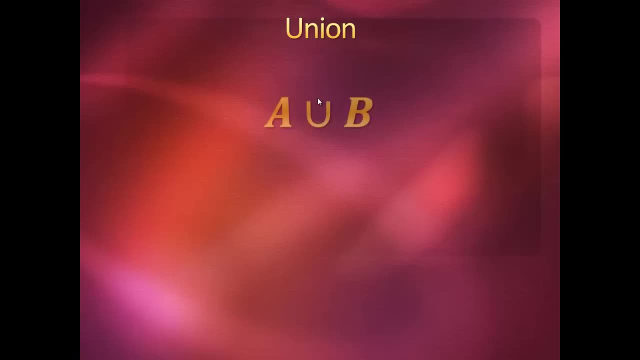 The second operator is called the union. This one's written like a right side up u, So we'd call this the union of a and b or a union b. The union is found by merging the two sets together, though, remember, each item can appear. 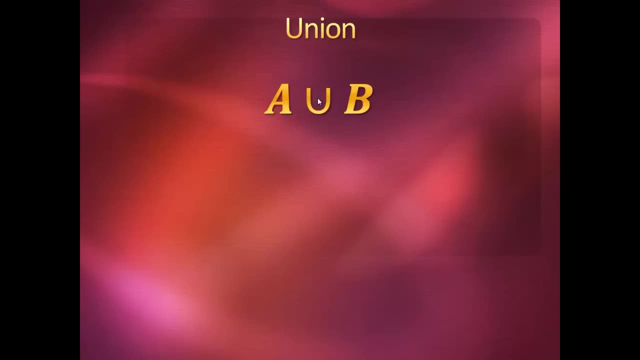 only once, so no doubling up on repeats. So what numbers do a and b have in common? We'd start with the elements of a, 1,, 2,, 3,, 4,, 5, and then put b's elements in. 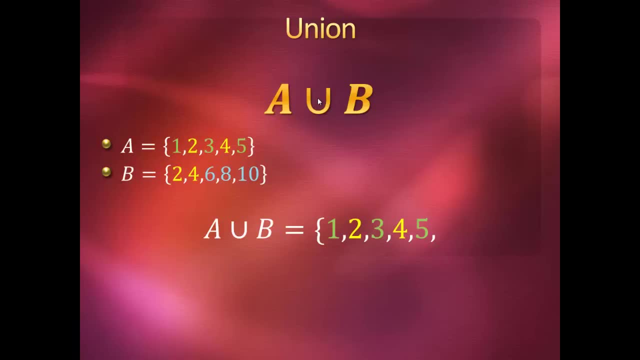 2 and 4 are already taken care of, so we just need to add 6,, 8, and 10.. Thus, the union of a and b is the set 1,, 2,, 3,, 4,, 5,, 6,, 8,, 10.. 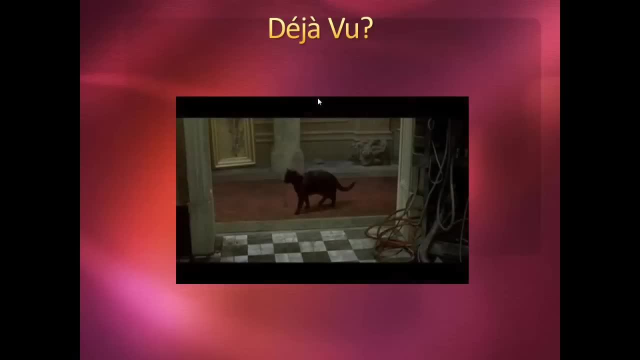 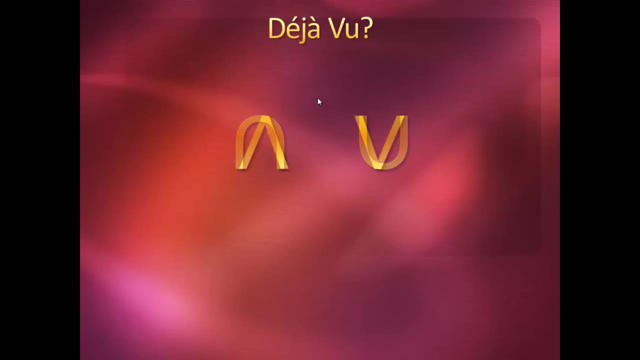 Now, some of you may have noticed something along the way. Does anyone else have a sense of deja vu? Well, I do. Where else have we seen symbols that look like this? The symbols for intersection and union kind of look like the symbols for conjunction and. 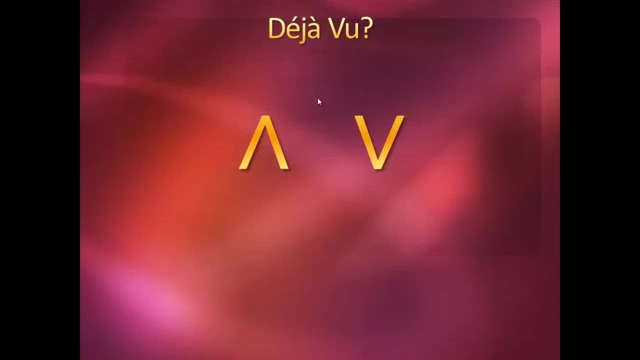 disjunction, don't they? Is this just coincidence? Well, let's re-examine what the intersection and the union really are and try to define them formally. Intuitive definitions are fine in math, but the real power comes from making formal definitions. 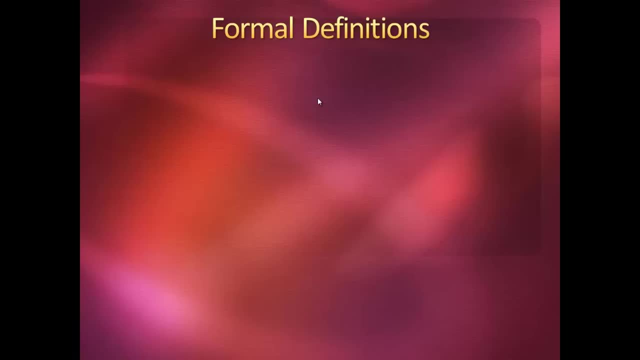 because that's where you can really see how things are related. So what is the intersection of a and b? Or rather, how do I know? if something is in the intersection of a and b, It has to be in a AND it has to be in b. 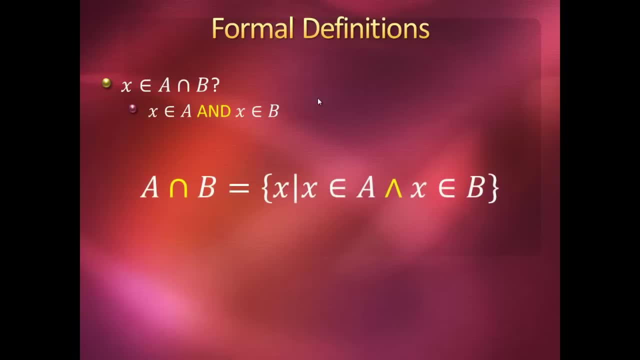 So, using set-builder notation, we can say that the intersection of a and b is the set of all things that are elements of a AND are elements of b. How about the union of a and b? Well, something is in the union of a and b, if it's in a OR if it's in b. 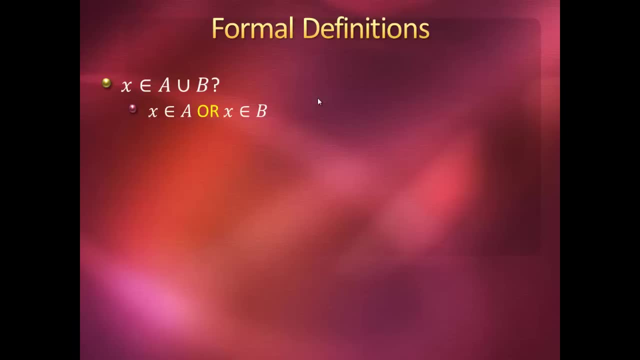 or if it's in both. So again, using set builder notation, the union of A and B is the set of all things that are elements of A or are elements of B, and that's an inclusive or. by the way, So it turns out, it wasn't a coincidence at all. 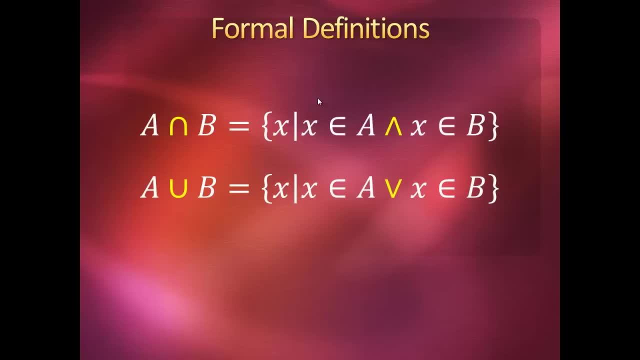 The intersection looks like a conjunction because it holds everything in A and B, and the union looks like a disjunction, because it holds everything in A or B. Gee, it's almost as if they intended that all along. Let's introduce another set C. This one will be 1,, 3,, 5, 7.. 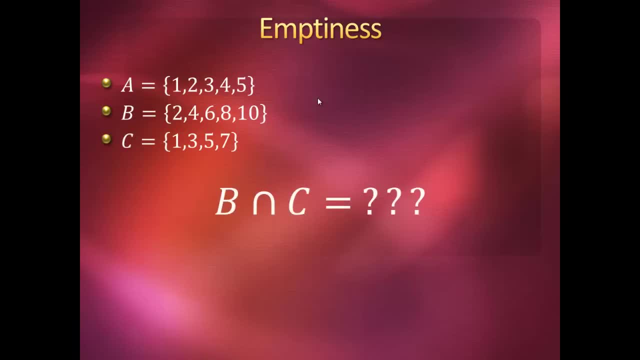 Now think what would be the intersection of B and C. They've got nothing in common. So that's our answer: A set with nothing in it. This is a special kind of set, we call the null set or the empty set, and there's two ways to represent it. 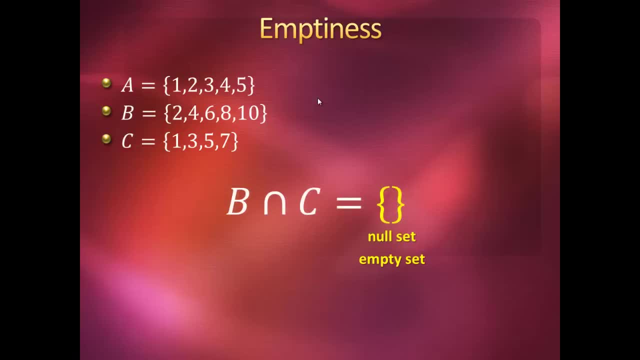 As a big O with a slash through it, or as an empty pair of brackets. So think of it this way: If we took a box and put in it everything that B and C had in common, then by the time we were done, the box would have nothing in it. 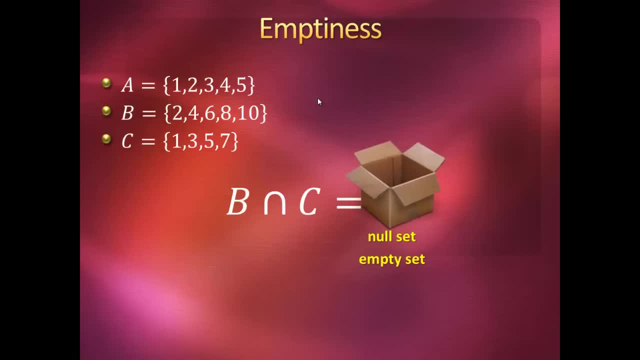 That box is an empty set. So another operator we can use on sets is called the difference. We write it using a backslash, not a forward slash, because those are used for something different. So the difference of A and B, which we might read as: 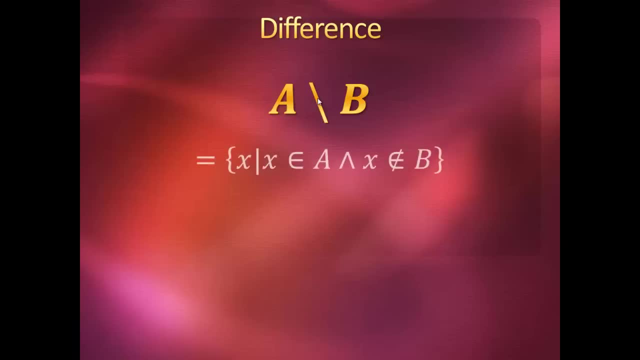 A minus B- Not really using a minus sign- is the set of everything in A that isn't in B. Basically, we start off with the elements of A and then take out anything that happens to also be in B. In other words, you take out the intersection of A and B. 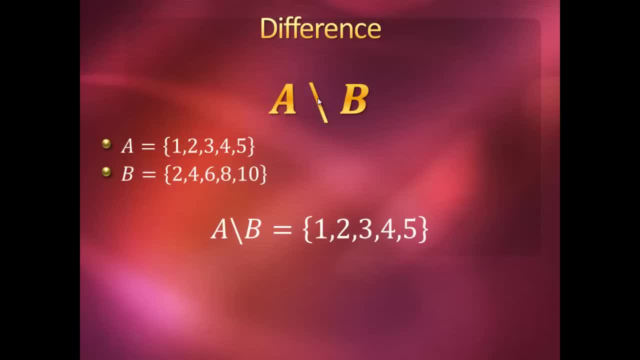 So, since the intersection of A and B is 2, 4, to find A minus B, we take that out of A, and thus we have 1,, 3, 5.. Similarly, for B minus A, we take 2, 4 out of B, and so we end up with. 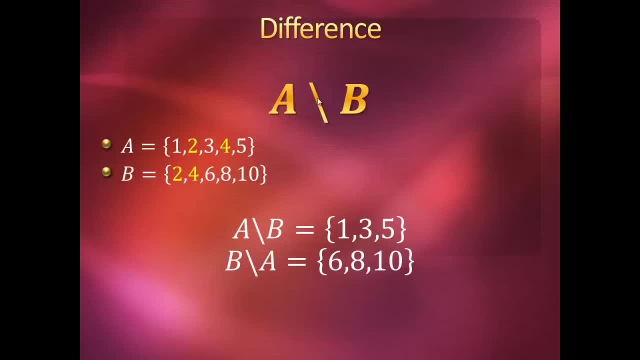 6,, 8,, 10.. From the difference of two sets we can define another operator called the symmetric difference, which we represent with a triangle or a capital Delta. The symmetric difference is what we get when we combine both set differences. In other words, the symmetric difference of A and B is just. 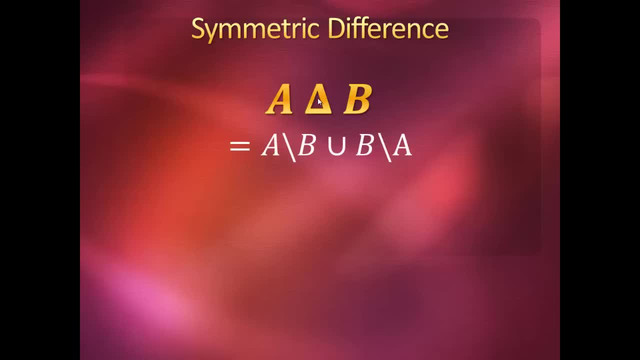 A minus B, union B minus A. So what does it mean for something to be in the symmetric difference? It would mean that it's in A or B, but not both Sound familiar. It's just like the exclusive disjunction, the XOR. See how the concepts of logic extend so perfectly to their analogs in 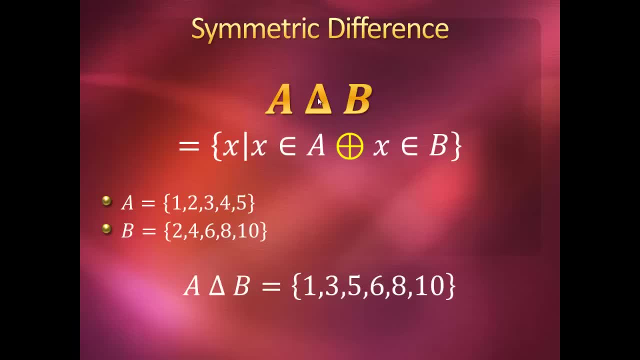 set theory. This is a common theme in this course and, in truth, a common theme in mathematics as a whole. A lot of concepts in math are related in ways that really clarify their meaning and make it a very rich subject, A tool we often use to more visually. 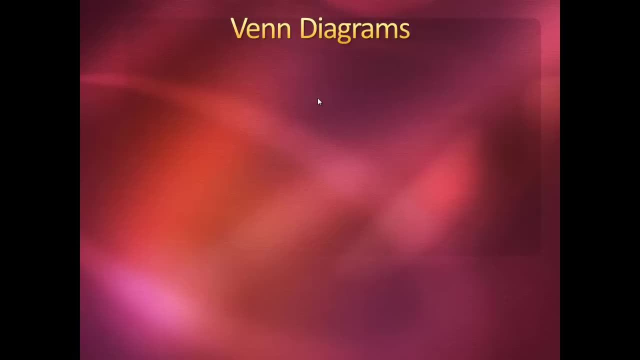 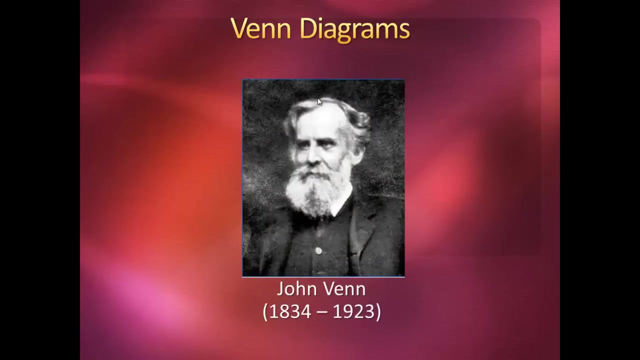 illustrate relationships between sets is a Venn diagram named for British logician and philosopher, John Venn. As it turns out, Venn created his diagrams first to represent logical relationships, but since the concepts of set theory are so analogous to those of logic, it's easy to make the transition In a Venn diagram. 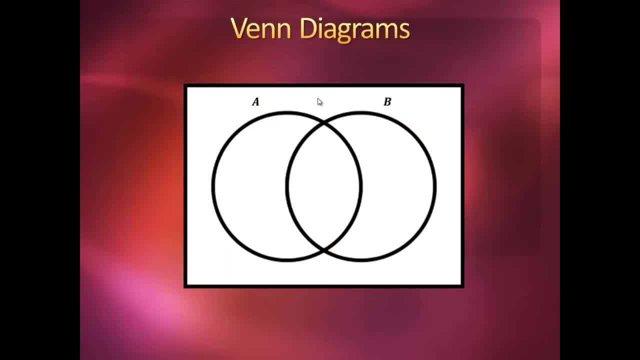 we use regions to represent sets. Usually the sets we start off with are circles. Then for the intersection, we shade everything the circles have in common. For the union, we shade both circles in. For the difference, we shade everything that's in the first set. 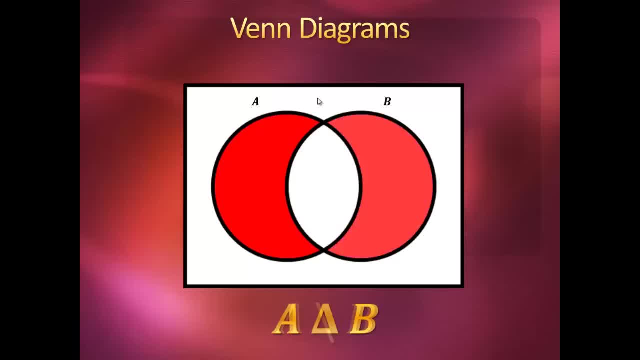 but leaving out its overlap with the second. And for the symmetric difference, we shade everything that's in one or the other set but not in their intersection. Using Venn diagrams helps us get a visual sense of what's going on. Moving on, let's take a moment to talk about. 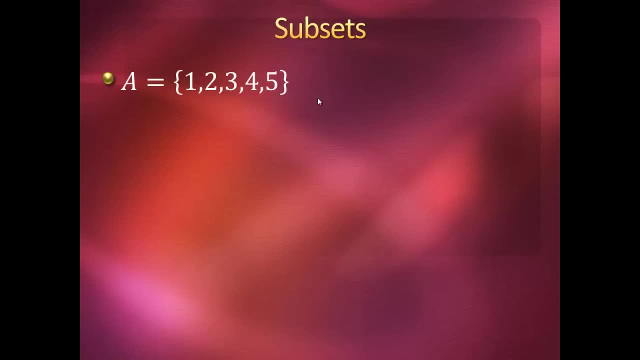 subsets. Suppose I start off with A and I take out some number of elements to make a new set which we might call D, Perhaps the set 1,, 2, 3.. We would say that D is a subset of A because it could be made by starting off with A. 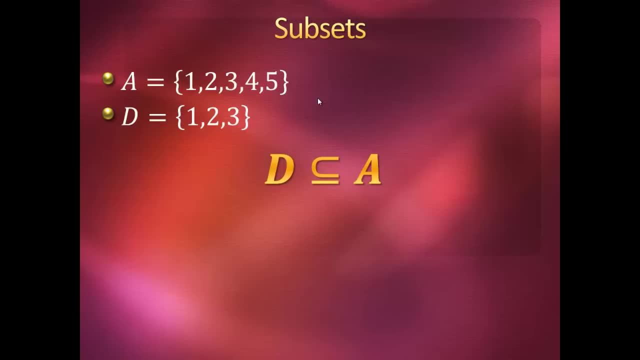 and removing some elements, The symbol looks kinda like a less than or equal to sign, but a little curvier. Notice that every element of D is also in A. This is actually how we formally define a subset. Saying that D is a subset of A means that if something is in D, 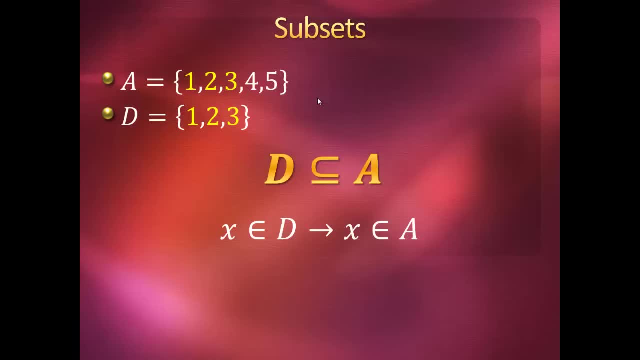 then it must also be in A Note that this means that the subset operator in set theory is the parallel to the conditional in logic. If E is the set 4,, 5, 6, then E is not a subset of A. There's a 6 in E, but there isn't one in A. 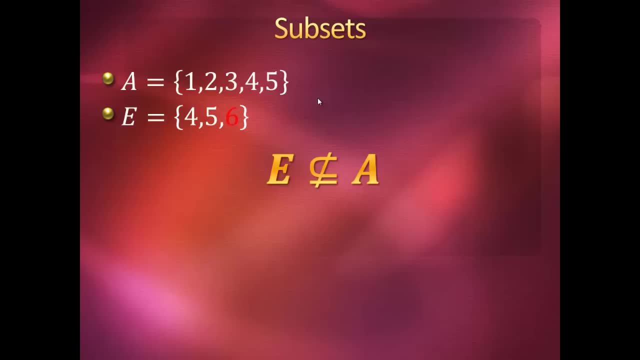 So we couldn't get E from A just by removing elements. By the way, if D is a subset of A, we can also say that A is a superset of D. The symbol to show this is just the normal subset symbol backwards, kinda like the greater than or equal to sign. We sometimes read this as: 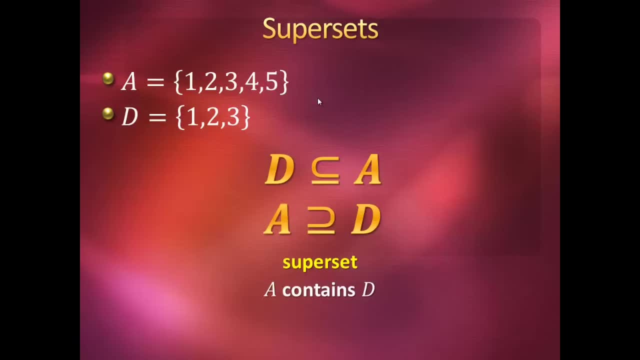 A contains D. Now for subsets. there are two special cases we may want to consider. First of all, is the null set a subset of A? We can tackle this two different ways. We can consider our original definition of a subset, the one involving removing elements. If we start off with D, then we can see that D is a subset of D. 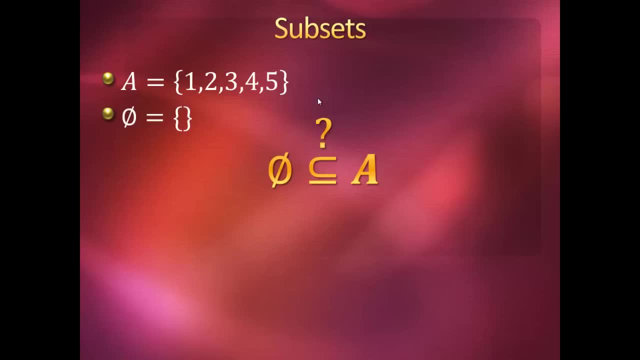 If we start off with A, we can get the null set by subtracting everything out of A. So by this definition of a subset we can conclude that the null set definitely is a subset of A. We can also consider the more formal definition, but this is somewhat trickier- For the null set to be a subset of A. 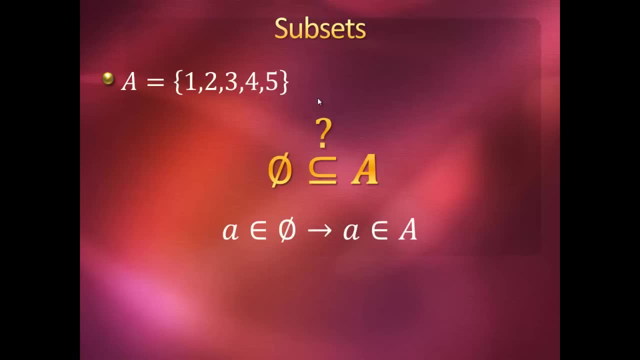 every element in the null set must be in A. How can that be possible if the null set has nothing in it? Remember that underlying the definition of a subset is a conditional subset. Let's take a look at the conditional statement. If X is in the null set, then X is in A. 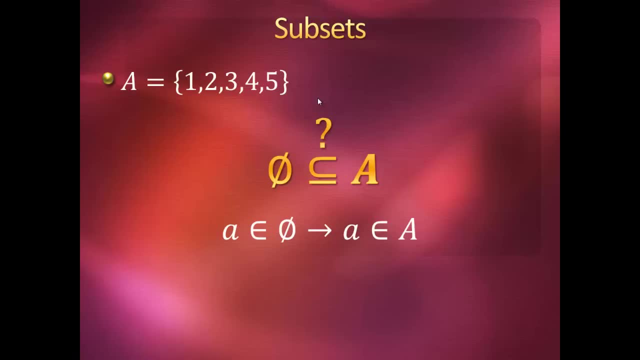 And the only way for this to be false is if there's something in the null set that isn't in A. Well, since there's nothing in the null set, we can be guaranteed that this is always true. Also, keep in mind that the conditional says nothing about what. 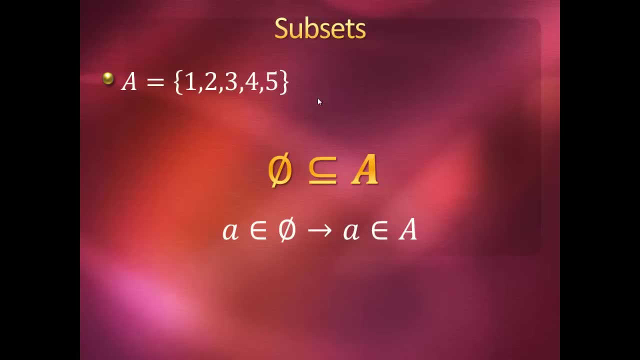 isn't in the null set, which is pretty much everything. So, as it turns out, it's true to say that everything in the null set is in A. In particular, we call this statement vacuously true, which means true in an empty sort of way. 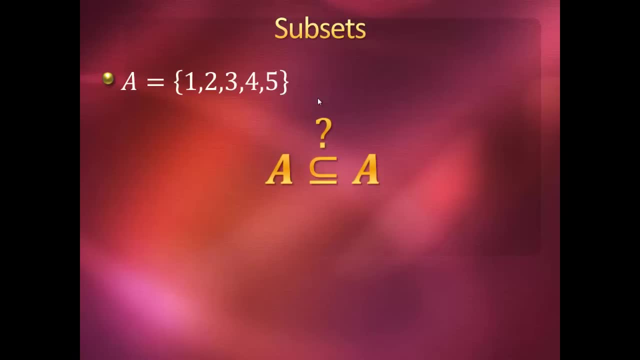 The second question we might want to ask is: is A a subset of itself? We could always start with A and then remove zero elements, but does that really count? Looking at the more formal definition actually makes the question more clear this time. If we pick any little A in big A, then must it also be in big A. 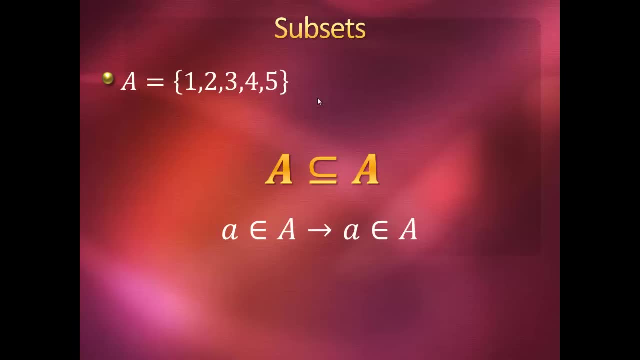 Well, of course, that's what we just said. So in that case, A is most definitely in the null set. It's definitely a subset of itself. In fact, given any set, A, the null set and A itself are called the trivial subsets of. 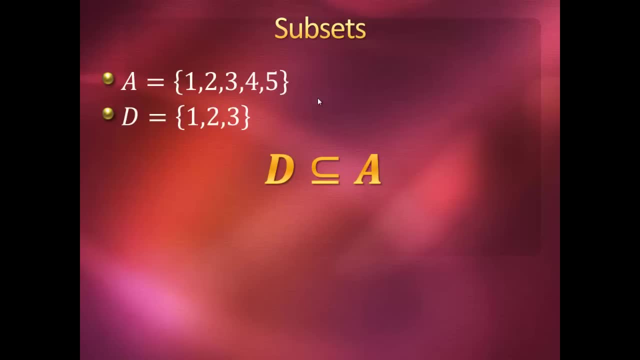 A. Now, if you're not satisfied with the idea of A being a subset of itself because it seems like you should have to remove something from A to be called a subset, I've got some relief for you. See the little bar under the subset symbol. 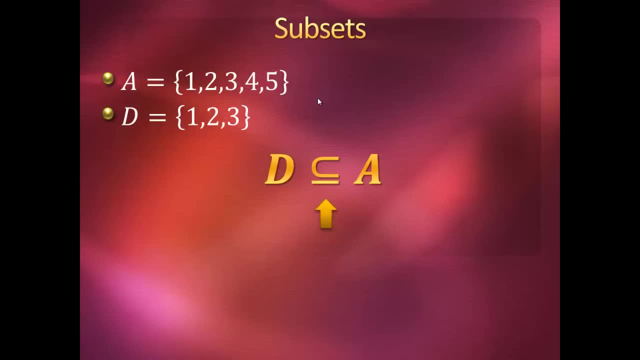 Remember how I said it resembles a less than or equal to sign. Well, wouldn't you think there would be some sort of analog to the just less than sign without the equal to? In fact, there is such an analog, just removing the bar. 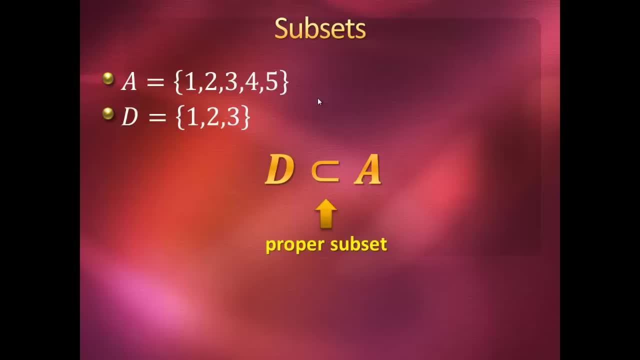 When we use this symbol, we actually say that we have a proper subset. So D is a proper subset of A, because D is obtained from A by removing at least one element of A. Every element in D is in A, but at least one element from A is not in D By this definition. 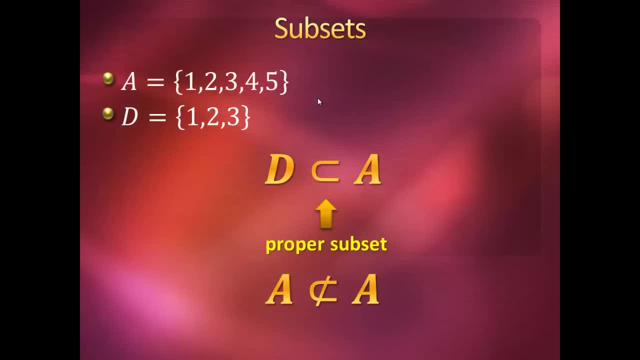 A is not a proper subset of itself. But wait, we just removed the equal to part of the subset symbol. What if we actually focus on the equal to part? That leads us directly into our next question. What does it mean for two sets to be equal? 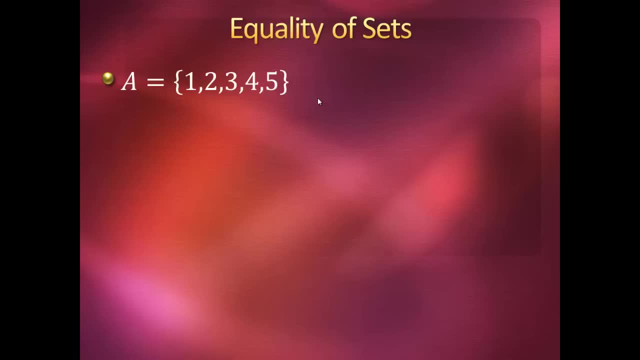 Well, it seems reasonable to say that two sets are equal when they have the exact same elements. So let's make a set F and we'll call it 1, 2, 3, 4, 5.. Looks just like A right. 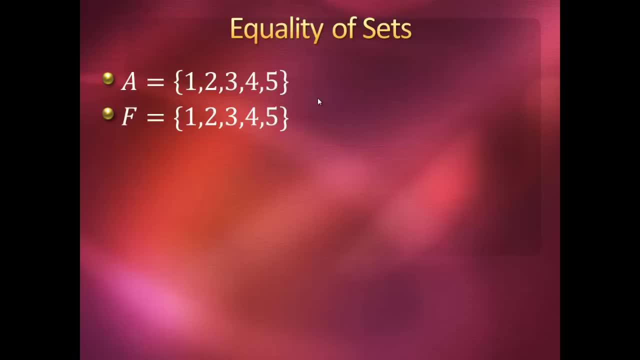 But are they equal? How do we check mathematically for sure? Well, luckily for us, we just learned about subsets, so this gives us a great way to attack this problem. First, we have to make sure that everything in A is in F. That's just checking to see. 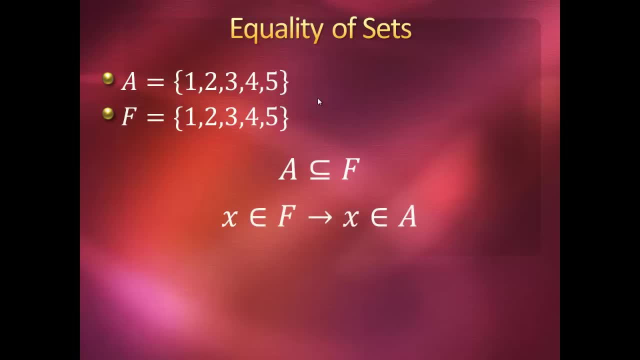 if A is a subset of F, Then we have to make sure that we haven't left anything out, that everything in F is also in A, And that's just checking to see if F is a subset of A. So A and F are equal. 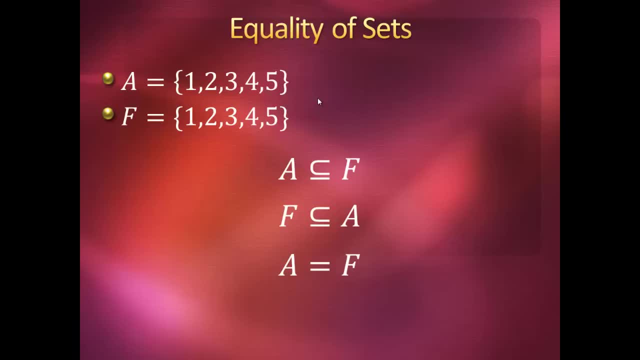 For example, if A is a subset of F and F is a subset of A, each one is a subset of the other. What's more, this shows how the equality of sets is just like the biconditional in logic. Proving a biconditional just required that we prove two conditional statements. 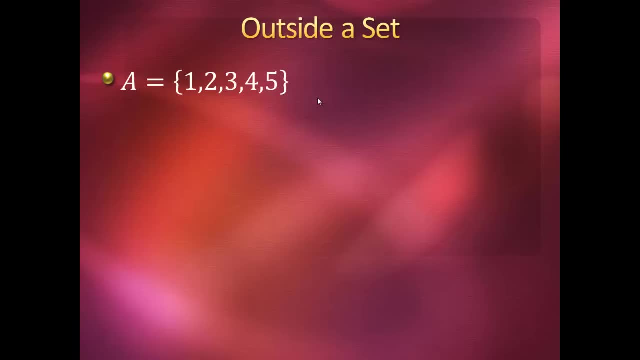 You may have noticed that there's a concept from logic we haven't established in Analog 2, the negation. Is there such a thing? We can talk about everything that isn't in set A, But that's quite a number of things. 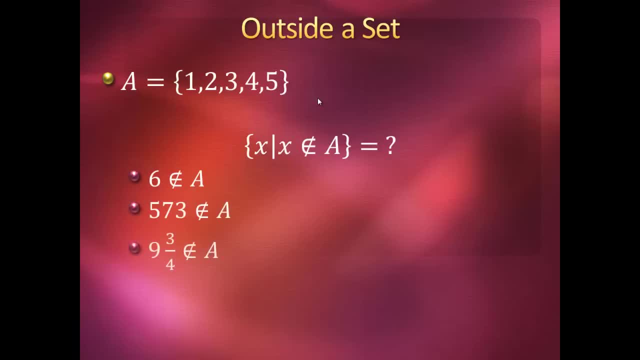 Six isn't in A, but neither is 573, or 9, 3 quarters, or pi or Swiss cheese. If we're talking about a problem involving only whole numbers, then we shouldn't particularly care about the fact that there's no Swiss cheese in A. 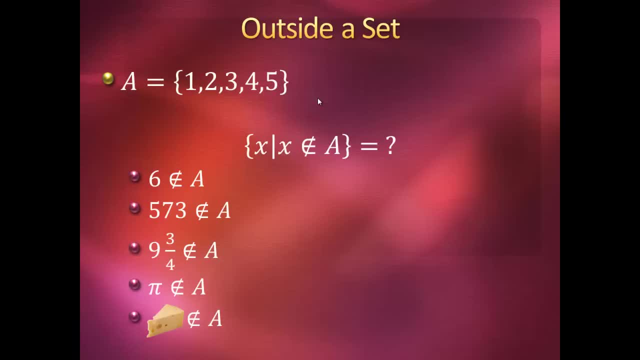 So, before we talk about what's not in a set, it may make a bit more sense to establish the idea of a universal set. The universal set is the set of everything we care about at the moment. The set of everything we care about at the moment. 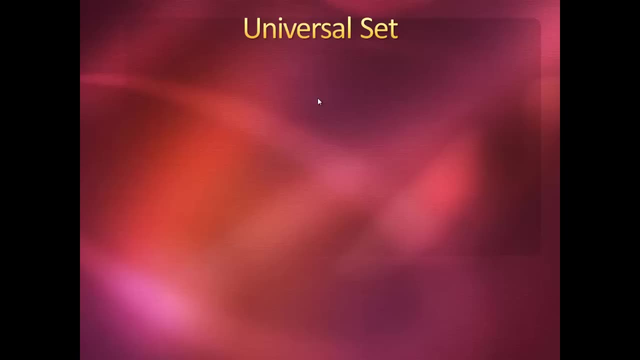 The set of all things that exist in the context of the current problem. Of course, this means that the universal set may be something different depending on what problem you're working on. Let's say that, for the purposes of this discussion, the universal set, which we write with a fancy- 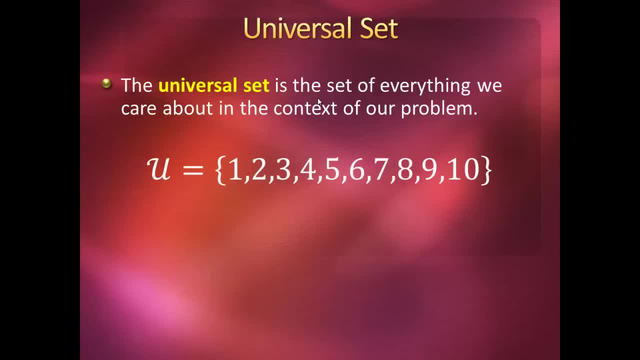 U- to keep it from being confused with the union- is the integers from 1 through 10 inclusive. Now that we've defined the universal set, it's time to meet the analog of the negation, called the complement of a set. Now that we've defined the universal set, it's time to meet the analog of the negation, called the complement of a set. 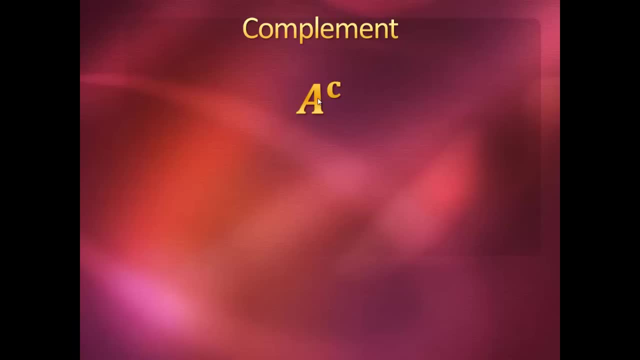 Now that we've defined the universal set, it's time to meet the analog of the negation called the complement of a set. The complement of a is written with a superscript C like this and is defined as everything in the universal set that is NOT in a. 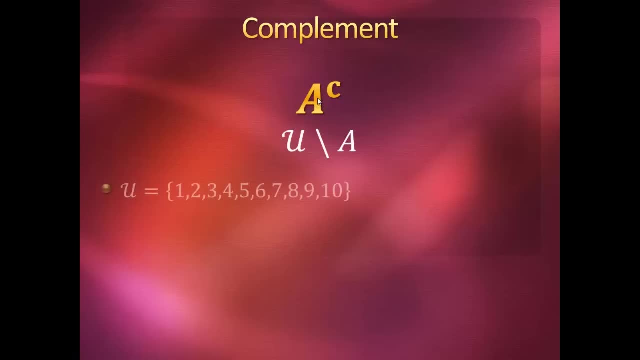 In other words U minus a. So in this case, a complement is the set. Now, the nice thing about the complement is that it has all the properties of the negation. So, for instance, can you guess what the complement of is? 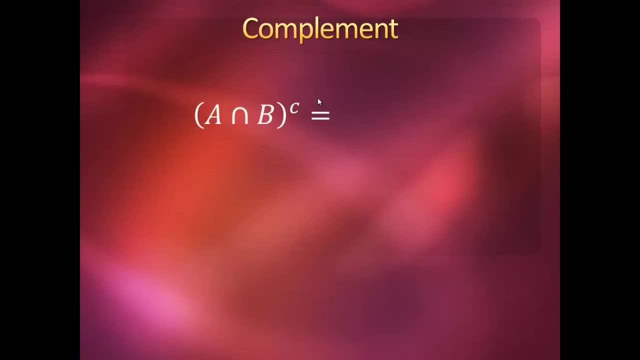 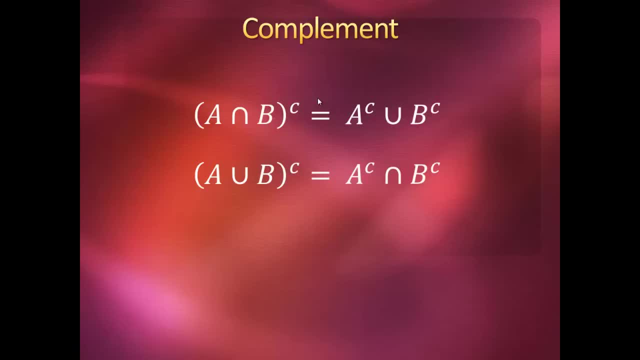 the complement of A union B is A complement, intersect B complement. How nice is it that De Morgan's laws automatically just work with sets, exactly as we hoped they would. By the way, see if you can draw some Venn diagrams to show De Morgan's laws at work. 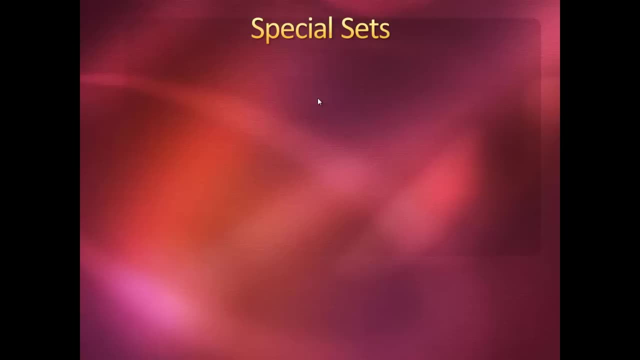 There are some sets that are used so often in math that they have special names of their own. You've probably encountered these before, but it helps to look at them in the context of what we've just talked about. The first set is the natural numbers. The natural numbers- 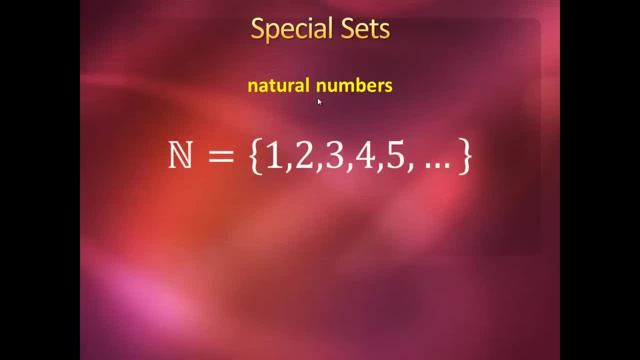 are the numbers we use to count objects 1,, 2,, 3,, 4,, 5, and so on. I won't list them all for hopefully obvious reasons. The set of natural numbers is usually denoted by capital N, Not just any capital N, but 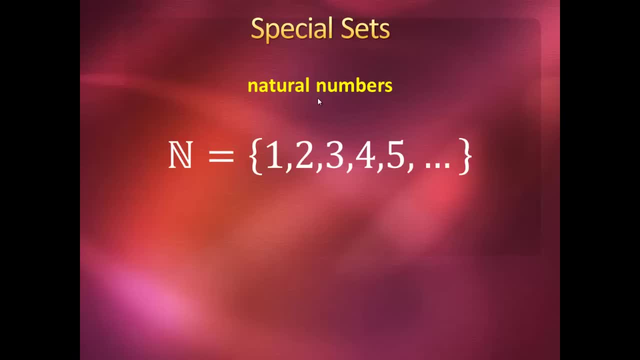 a double-struck N, where we double some of the lines. This style of writing is sometimes called blackboard bold. Now, a question you may have is: is zero a natural number? We can talk about zero objects, can't we? Well, in grade school it's often taught that zero. 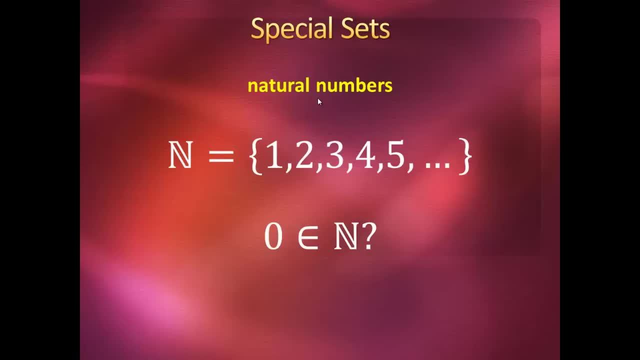 is not a natural number. But in reality mathematicians don't really have a consensus on whether zero should be included. Sometimes it's convenient to assume that N includes zero. Other times it's convenient to leave it out. Sometimes it doesn't even matter as a problem that uses one can sometimes 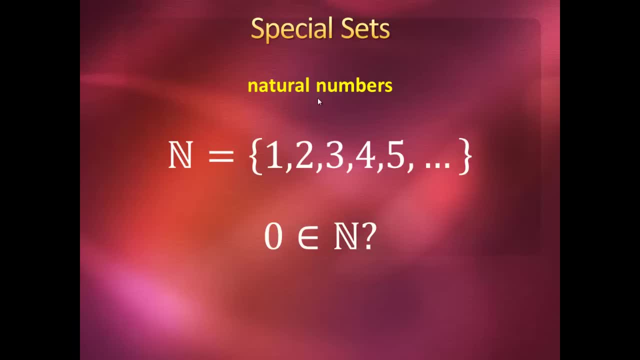 be just modified to use the other. In this course, we'll assume that N does not include zero. If we do need to include zero, we'll specifically say so by saying N union zero. The next set is the integers. The integers do include zero for a fact. For example, we'll say N union zero. The next set is the integers. The integers do include zero for a fact. For example, if we do say N union zero, we'll say zero for a fact. If we do say N union zero, we'll say: 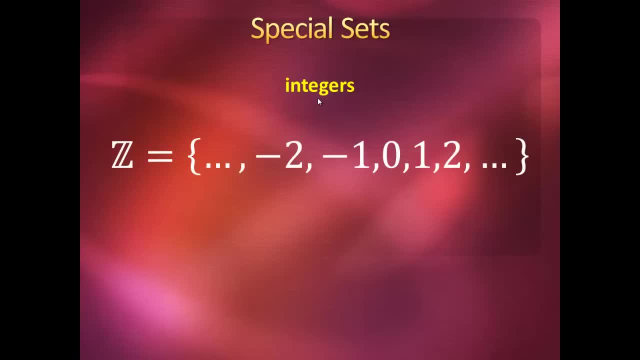 N equal zero. We will then use the negative numeric numbers, so N union zero. Instead of a negative number being negative, we'll say N equal zero. In this case we can look to the positive number of the integer, and they include the. 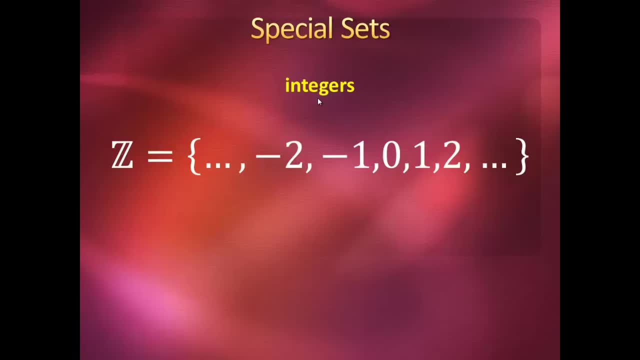 negative counter parts of the natural numbers: negative one, negative two, negative three, and so on. We represent the integers with a double-struck capital, z. This may seem a little strange at first, but it's because it's short for the German word Zahlen, meaning numbers. 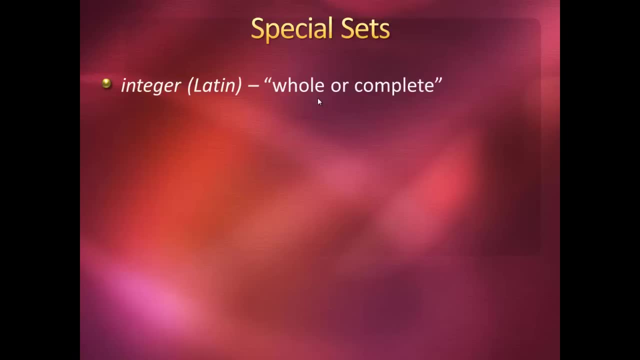 Perhaps because Kanter was German. The word integer in Latin, spelled the same way, actually meant whole or complete, which makes sense, because all the integers are whole numbers. We have number N integer, which shall be double or complete, because all the integers are whole numbers. and it's also where the English 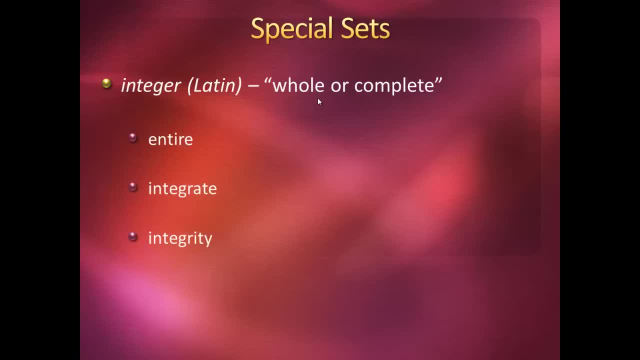 words entire, integrate and integrity come from. After the integers is the rational numbers. These are not the numbers that are capable of thinking. Rather, they are all numbers that can be expressed as fractions or ratios of two integers. hence the name rational. The letter we use this time is a double. 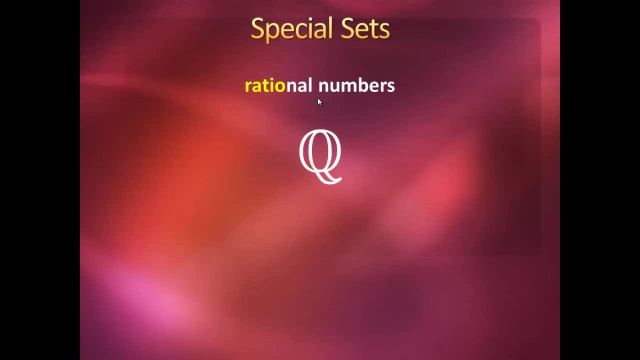 struck capital Q, which again seems strange, but this time it's because it stands for quotient, the result of a division. Listing them in order is much harder, though, as we'll see later in the course, there actually is a way to do it. 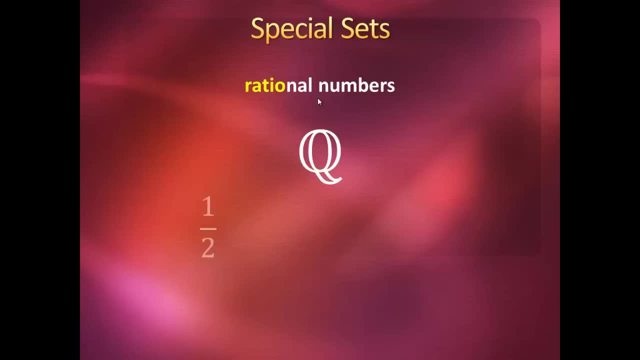 So instead we'll look at some examples. 1, half is a rational number because it's the ratio of two integers: 1 and 2.. Negative 3, fourths is another one: the ratio of negative 3 to 4.. 5 is a rational number because it's the ratio of two. 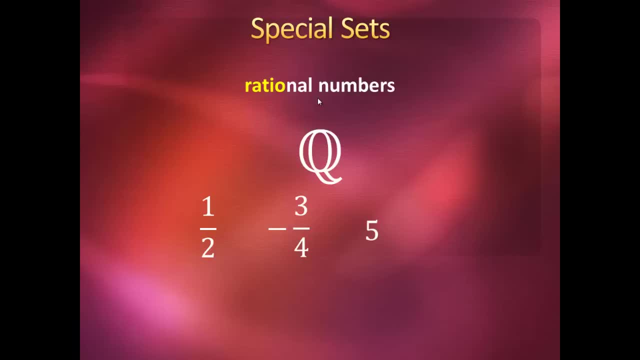 integers 1 and 2.. Negative 3, fourths, is another one: the ratio of negative 3 to 4.. But wait, isn't that an integer? How can that be a fraction? Well, we can write it as the ratio of 5 to 1, so it is in fact in Q. Also showing up in Q are 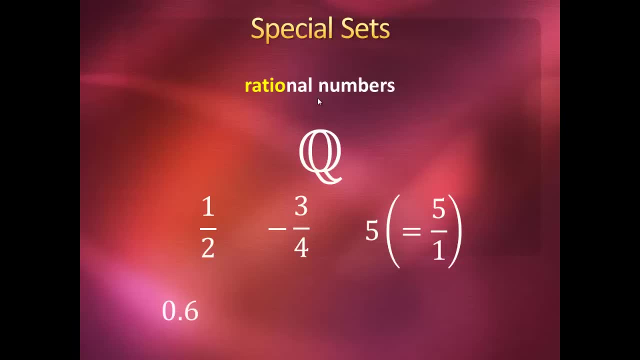 terminating decimals, such as 0.6,, which can be written as 3 over 5, and infinitely repeating decimals, such as 0.333, repeating which can be written as 1 over 3.. Now, even though the natural numbers are quite numerous, there's still quite a few numbers left out, Lots of. 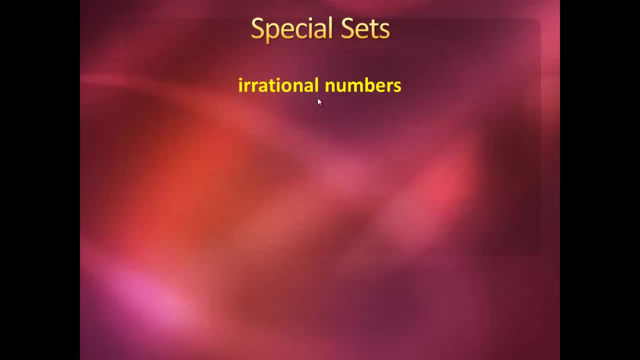 numbers can't be represented as a fraction. These numbers are called irrational numbers When written in their decimal expansions. irrational numbers will go on forever after the decimal point, but without ever repeating. Some good examples of irrational numbers you've probably seen before are pi, e and. 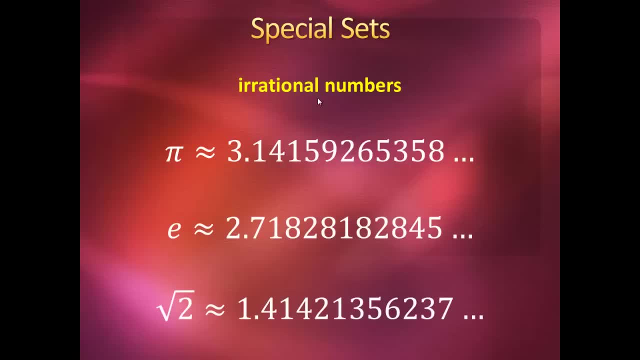 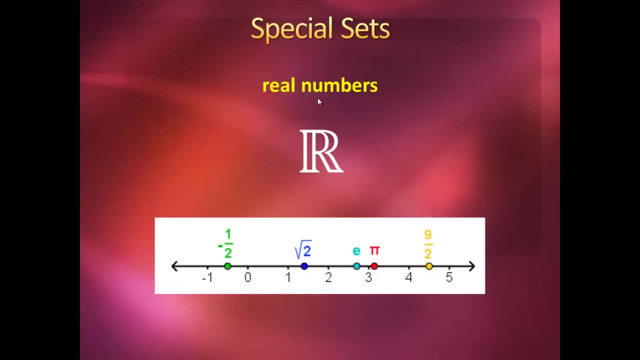 the square root of 2. If we add these irrational numbers to the rational numbers, we get a more complete set that we call the real numbers, represented by a double struck capital R. The real numbers complete the number line. so a good way to think about it is, if you can point to, 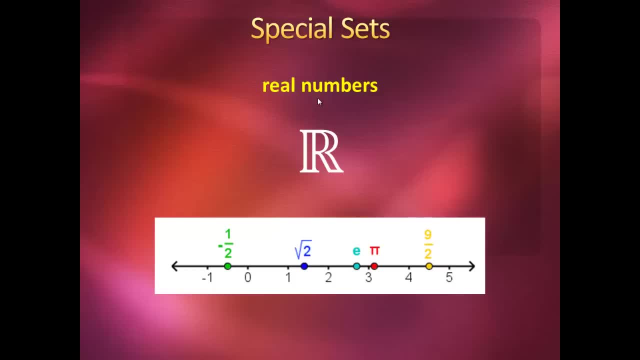 it on the number line, it's a real number. The irrational numbers don't usually get their own symbol, so they're often represented as just R minus Q. The real numbers are one of the most convenient number systems to work with mathematically, and we'll be devoting a few lectures just to study their 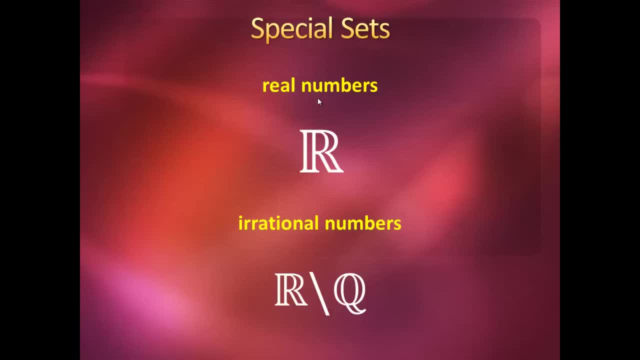 properties. However, there's one more, even larger set of numbers we often deal with, called the complex numbers written as a double struck capital C, which are all the numbers that can be written as a plus b times i, where i is the square root of negative 1.. There are other, even larger, 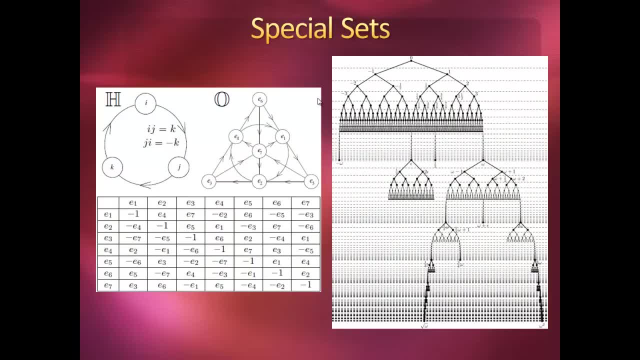 sets of numbers that have their purposes in various fields of math and physics, but there's no need to get into them here. What is important is that you understand the sets above and know their names and symbols, as they're ubiquitous in pretty much every math class you will. 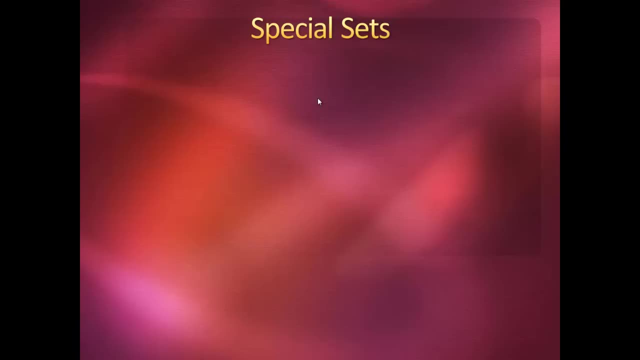 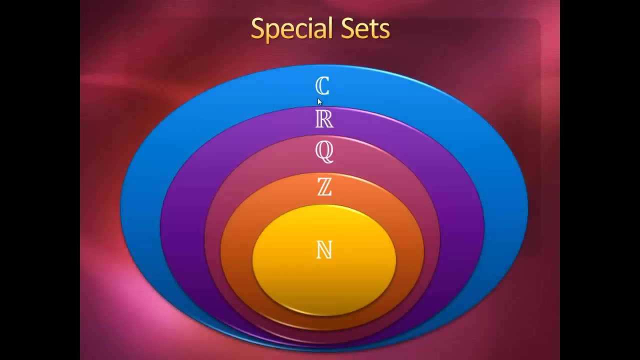 take from here on out. Something you may notice is that these sets actually have a rather nice hierarchy. The natural numbers are a subset of the integers, which are a subset of the rational numbers, which are themselves a subset of the real numbers, which are finally a subset of the complex numbers. One last, 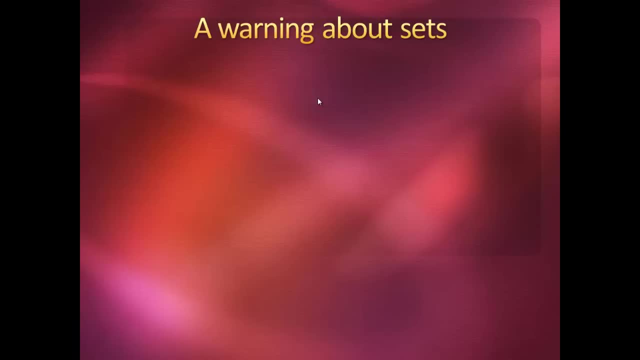 thing I'd like to go over about sets. We've said that sets can contain just about anything. The key words here are just about. There's one restriction that we have to be careful of when talking about set theory: A set cannot contain other sets. Now, this may seem strange to you. 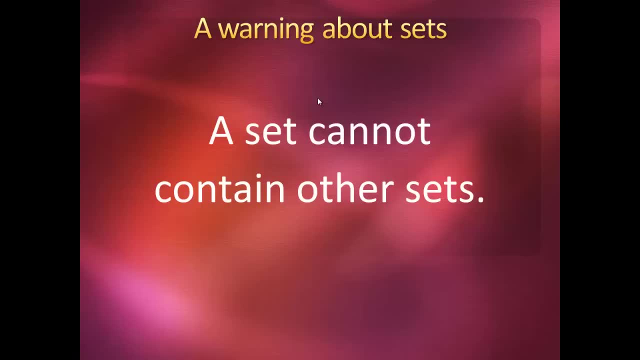 Surely there's nothing stopping us from making a set of sets, is there? Well, that's what mathematicians thought about sets for a long time, until someone came along, as they always seem to in the history of math, and turned their world. 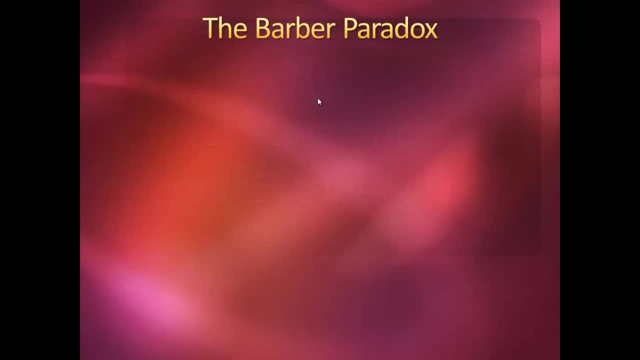 upside down. Imagine the following scenario: Suppose you live in the town of Seville, where there lives a man who is the only barber in town. Every man in this town keeps clean shaven by doing exactly one of two things: He either shaves himself, 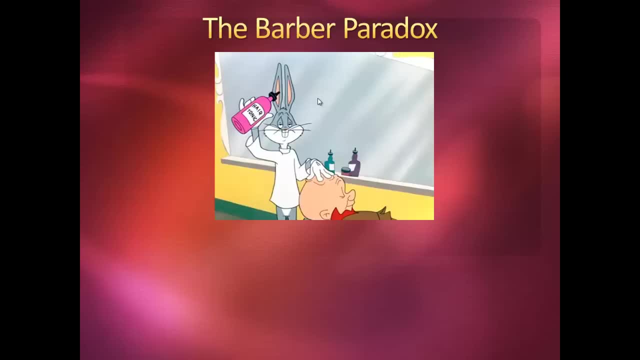 or he goes to the barber, but not both. In other words, the barber shaves those, and only those, men in town who do not shave themselves. The question is: who shaves the barber? Think about this for a second, but not too long, because it's quite 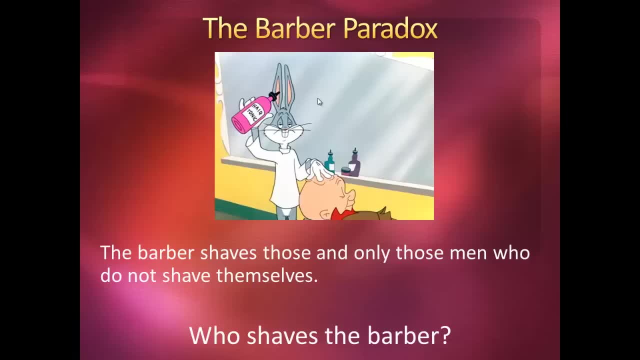 painful to think about. If the barber does shave himself, then he is one of the people in town who does not shave himself, But those are precisely the people he does shave. On the other hand, if he does shave himself, then he is not one of the people who 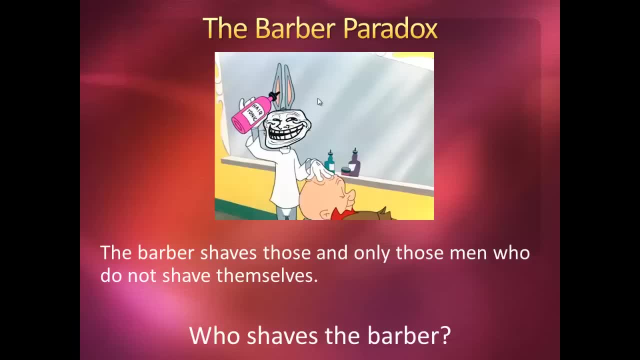 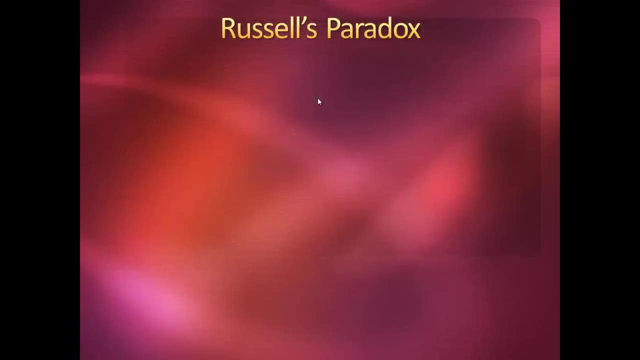 shaves. You see how twisted this becomes. This is a classic paradox, a situation that contradicts itself. Imagining this paradox will help you understand the paradox that puzzled the minds of set theorists. The paradox we're about to talk about is known as Russell's Paradox, as it was found by British mathematician and philosopher Bertrand Russell.